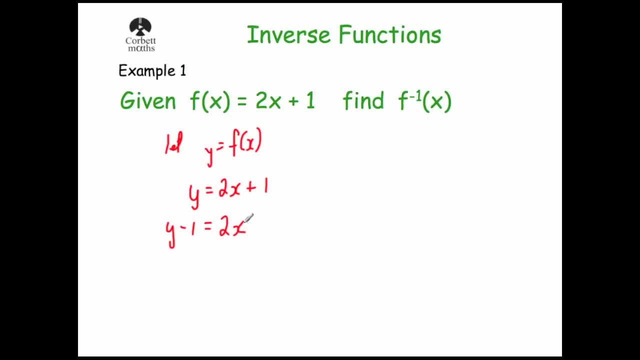 sides. So we're going to get y minus one equals two x. Then we're going to divide both sides by two. Obviously, we're trying to make x a subject here. So y minus one divided by two equals x, And that's it. So this would be the inverse. 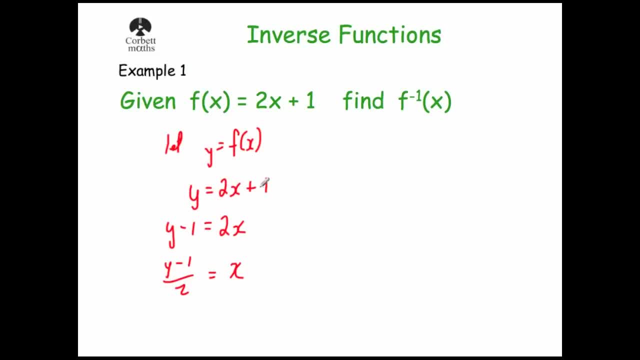 function. So, to get from x to y, you would times it by two and then add one. To go from y to x, you would take away one and then divide by two. So this is the inverse function. Now the way we write our answer is we write f minus one of x. Now what we're going to do is we're going to change this. 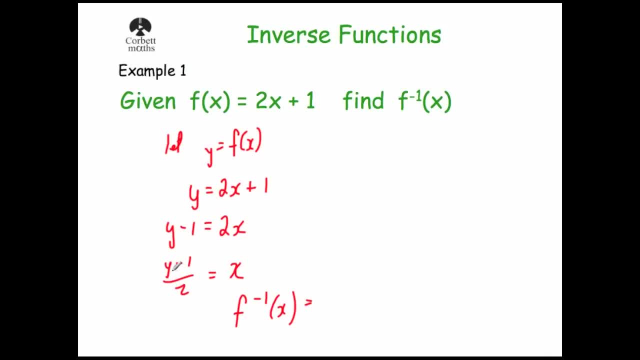 answer into. back to x's. Okay, we want to use the same variable. So instead of y minus one divided by two, we're going to write x minus one divided by two. Okay, and that's it. So if the function of x is two times x plus one, the inverse function would be x minus one and then divided by two. 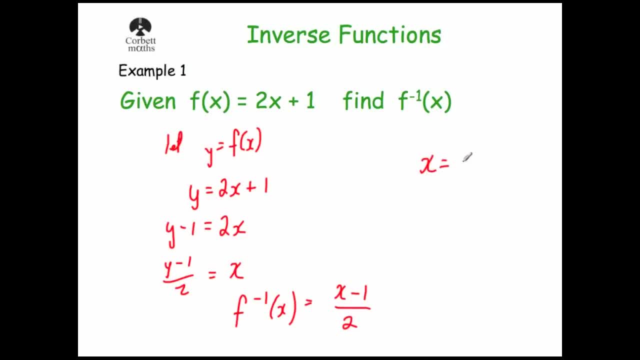 Let's try it out. Let's just say, for instance, x is equal to- I don't know- ten. So two times ten is equal to twenty plus one is twenty one. So if we want to go backwards, let's put twenty one into here. So twenty one minus one is twenty. divided by two is ten. So it does work. So that's how I. 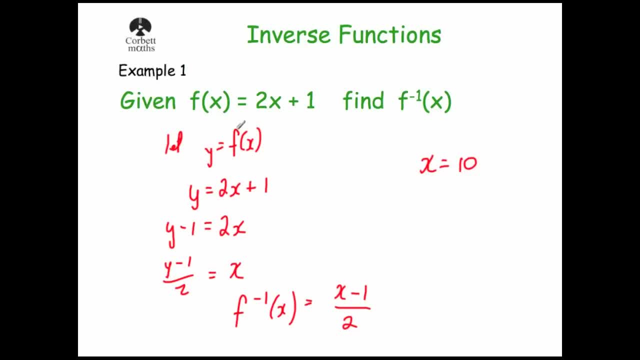 would approach an inverse functions question. I let the function they give me in the question be. I then make x a subject and then that would give me the inverse function. I would then write down f minus one of x or whatever it might be, g minus one of x and then write it equal to the function. 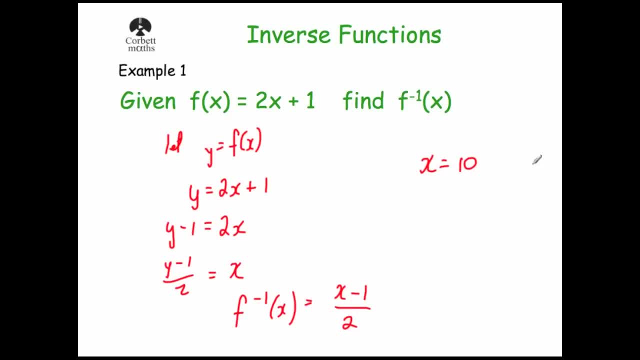 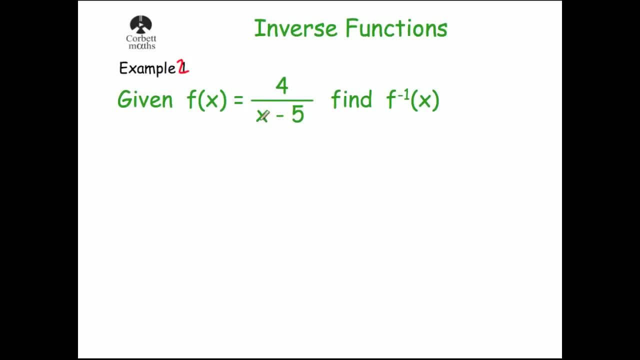 but change the letter from y back to an x. That's it. Let's have a look at another example. Okay, so let's have a look at example two. So example two says: given f of x equals four over x minus five, find f minus one of x the inverse function of x. So remember our approach: we let y equals f of x. 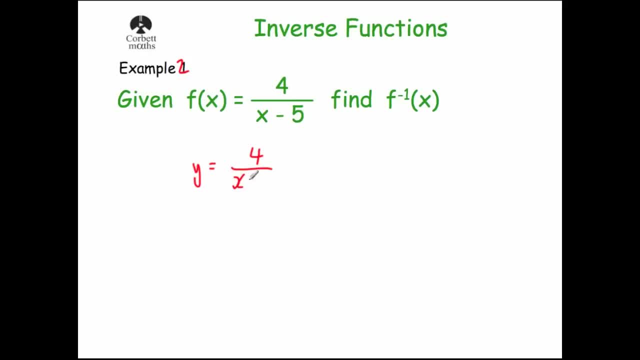 so we write: y equals 4 over x minus 5. now we want to make x a subject. now we've got a bit of a problem here. x is under the denominator, so we're going to need to multiply both sides by x minus 5. doing that, we give me y bracket. x minus 5 equals 4. now, remember again, we want to make x a subject. 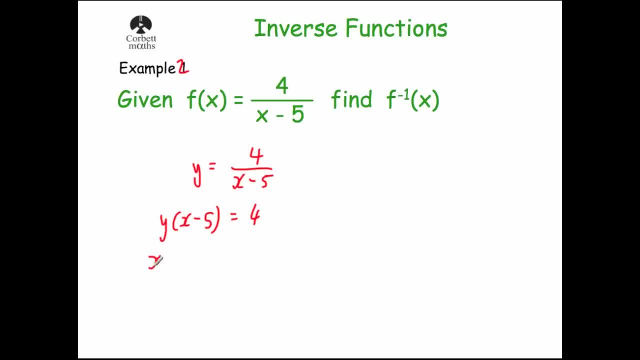 so we don't want it in the brackets. we're going to need to multiply the bracket to get x? y minus 5 y equals 4, and to make x a subject, well, let's add 5 y to both sides, so x? y equals 4 plus 5 y. 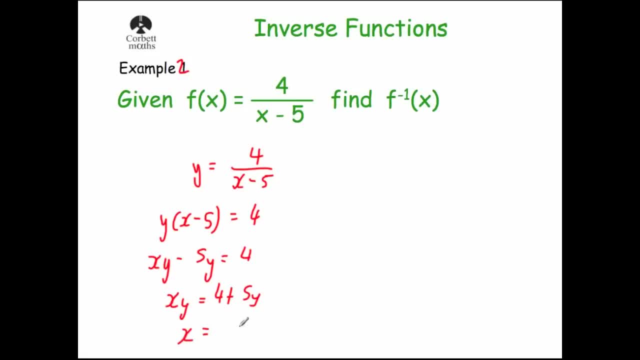 and we want to divide by y. so we're going to get x equals 4 plus 5 y over y. now that means that x is equal to 4 plus 5 y over y, or we could divide through by y. so what that would mean is we get 4. 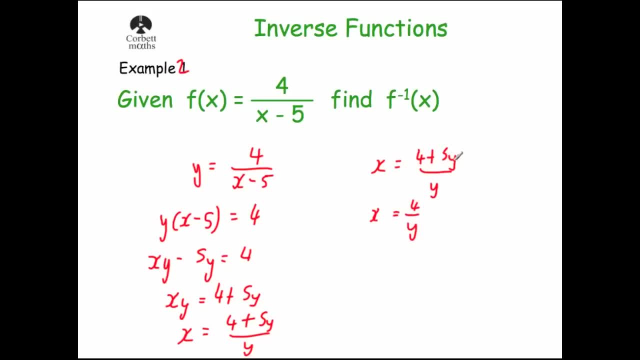 divided by y, which is 4 over y, and we would get 5y divided by y, which will be plus 5.. I'm going to use this version here: 4 over y plus 4 over y plus 5.. So that's it. we've made x a subject. now, remember, if we want to want to write. 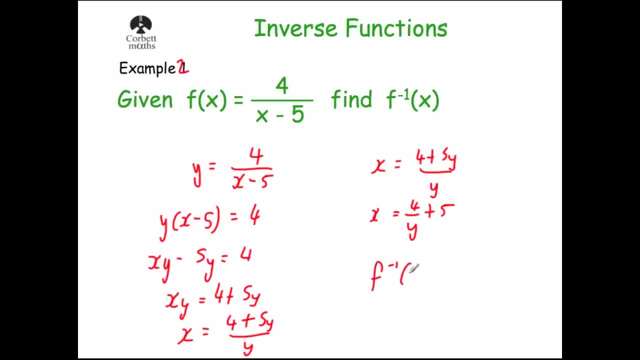 that in the f minus 1 notation. so we're going to write f minus 1 of x and we're going to replace the y with an x equals 4 over x plus 5, and that's it. that's the inverse function. So if you've got, 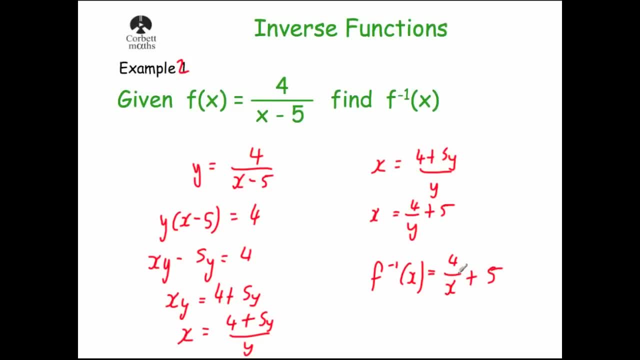 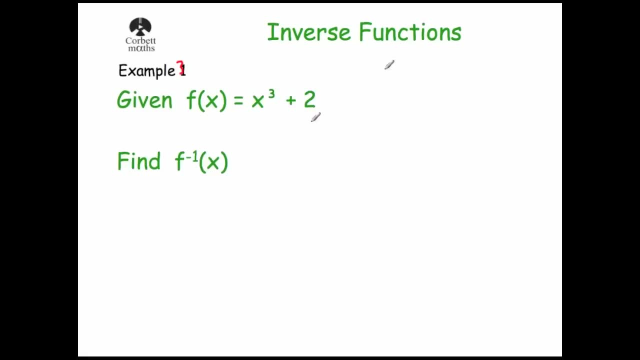 a function: 4 over x plus 5. the inverse function would be 4 over x plus 5.. Okay, so it says: given that f of x equals x cubed plus 2, find f minus 1 of x, find the inverse function. So again that's the function in the question: equal y. so y equals x cubed plus 2. 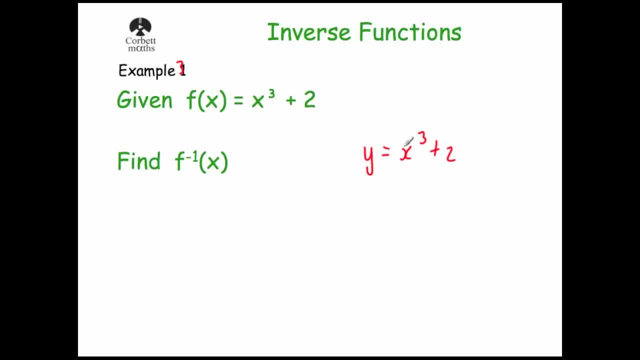 and make x a subject. so we're going to subtract 2 from both sides. so y minus 2 equals x cubed. and now we're going to cube root both sides. Now be careful: if it was a square to do with what value you're going to get. So if it was a square, then you're going to get x cubed plus 2. 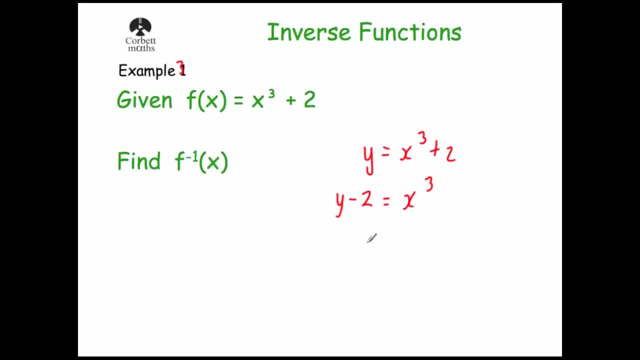 of x and y can work and that's more of an a-level topic, and this video I've made today is focused on the sort of the new GCSE style questions, which I don't think would include too much detail in terms of domains and ranges. Again, if you're doing GCSE maths, don't worry too much about what I'm. 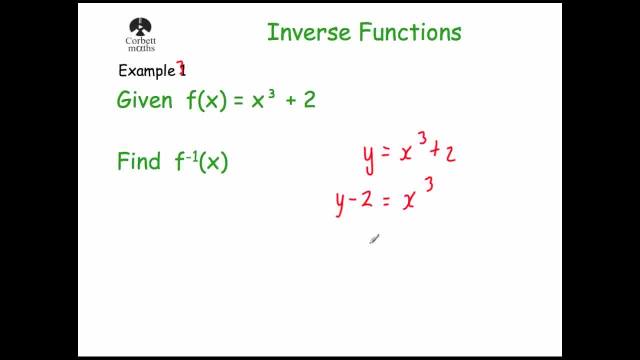 saying at the minute, but just be aware that if you're doing a-level maths, there's another video on corporate maths you'd want to watch. And then we're going to cube root both sides here. so the cube root of both sides would give me the cube root of y minus 2 equals x. Now, remember, we want.